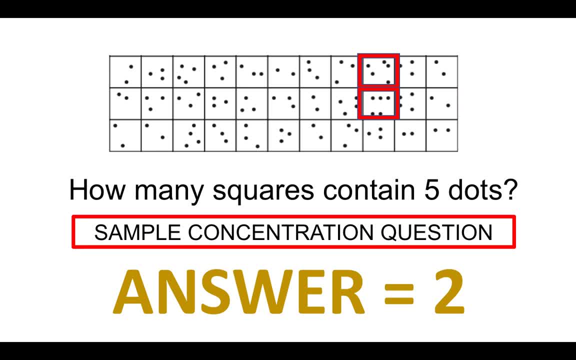 you question one, and then I'm going to give you the answer, then question two give you the answer, and so on and so forth. So you'll get a little bit of a break between each one And, trust me, you're going to need it. Now. I have placed a timer on each page, So please. 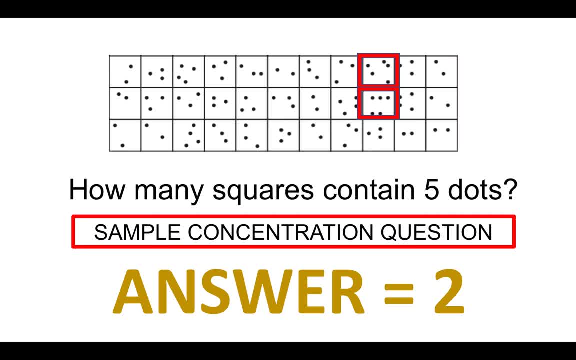 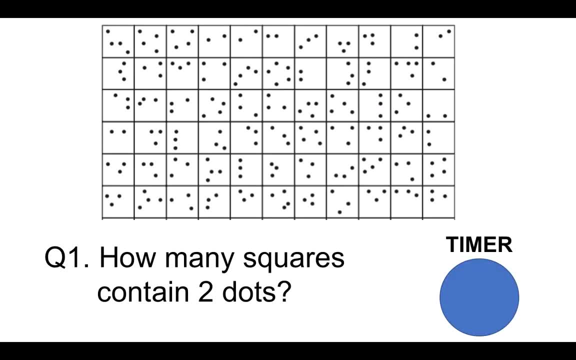 do work strictly within the timer. Okay, so let's get started. So get your eyes ready, Make sure there's no distractions around, And the first question is: how many squares contain two dots? And you've got until the timer runs down to answer this question: How many? 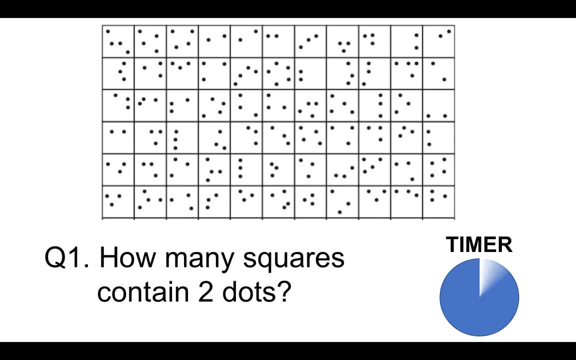 squares contain two dots. Okay, Now, if you got to the end of this within the timer, you've done really well. Now, if you want to get to the end of this, just remember there's a little bottom line there. Okay, trust me. 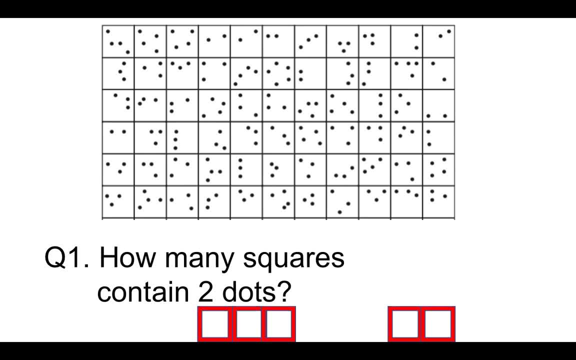 you've got really good concentration skills. Furthermore, if you get it actually right, then you've done even better. So let's take a look now at the answer to this one. So if we go line by line, we can see that there's two there. There are five across the first. 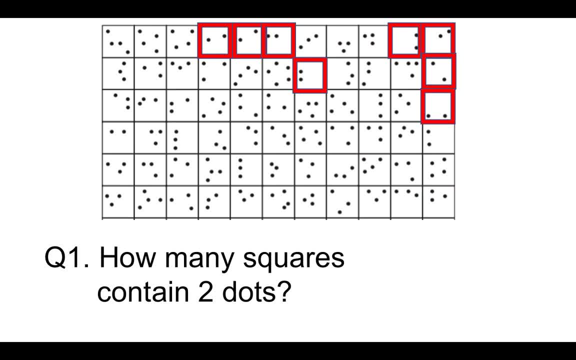 line, There's just two across the second line, There's one across the third line, There's two across the fourth line. So in total, and that's all there is. there are none across the final two lines. So the total number of squares that contain two dots equals 10.. Now, 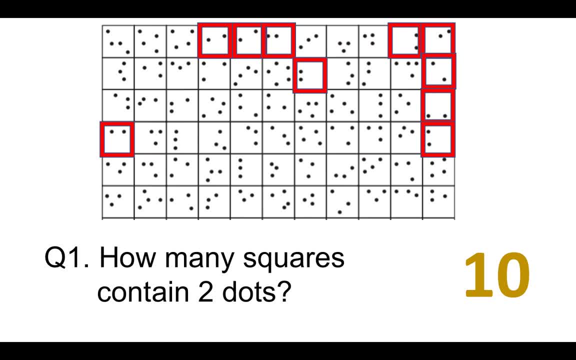 Now, if you got that right, well done. Let's get a little bit harder now. So then the next one. you'll have a little bit longer, but you'll have more work to do. So question number two: and don't forget to work strictly within the timer. How many squares contain? 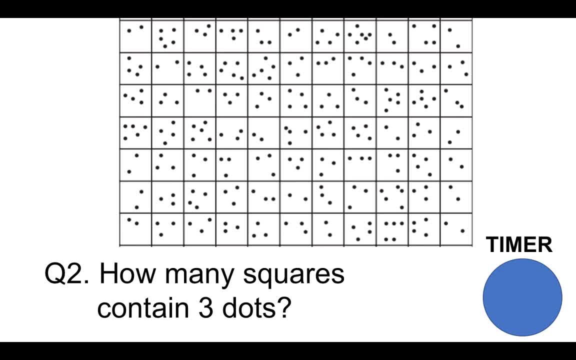 three dots And you've got the time until the timer runs down to complete this question. Okay, Okay, Now again. if you got to the end of this one in particular, you've done really well, because you will have noticed that there's more squares with dots in them. This one is: 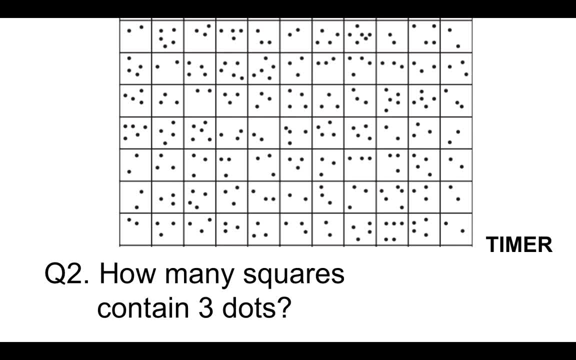 a tough question and you didn't have that long to work through, But if you got it right, then you've done really well. At this stage, please put in the comments section below what you think of this test, whether you find it easy or hard. Personally, I find it quite. 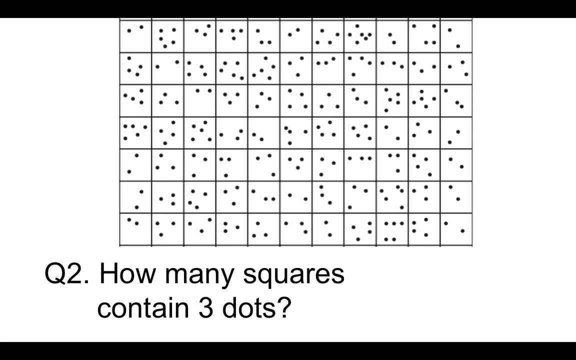 difficult. Let's see if you got question two right, How many squares contain three dots? Okay, So it's just two across the top On the second line you'll see this five. Then if you move down to the third one, then 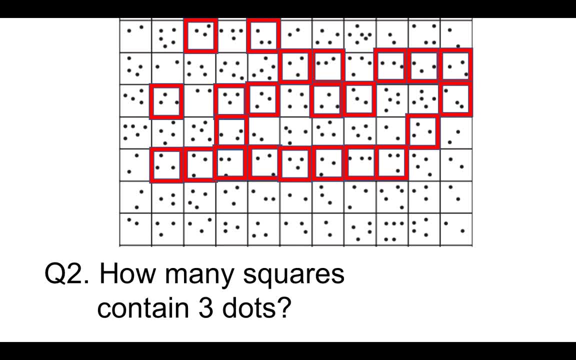 you've got six, two in the next line, and then you've got a whole raft of them together. You've got one, two, three, four, five, six, seven, eight together. Then you've got six on the next line and five on the bottom, given a total of 34 that you had to find, And again, 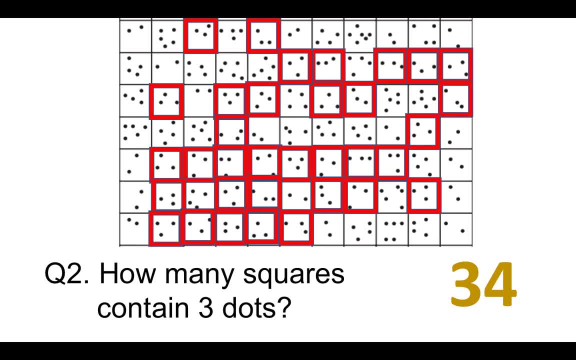 if you've got that right, you have done tremendously well and you deserve a pat on the back. So give yourself a pat on the back. Let me know in the comments section how well you're doing. We're now going to move on to another one. Okay, So we're going to move on to another one. 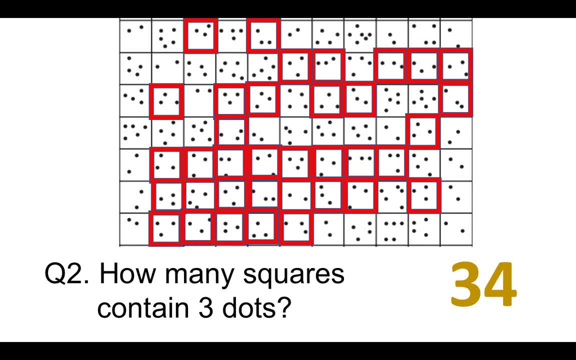 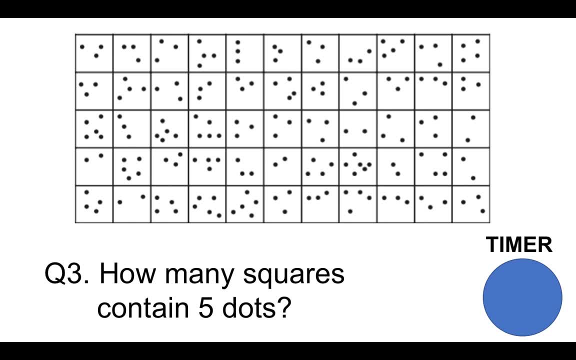 Okay, So get yourself ready. Hopefully your eyes and your brain are still keeping up with this. Next question: How many squares contain five dots? And again, you've got the time until the timer runs down to get this one correct. 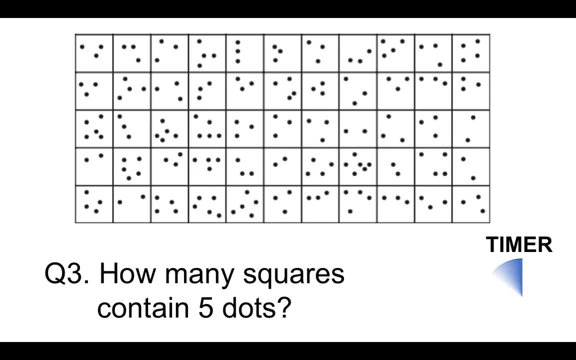 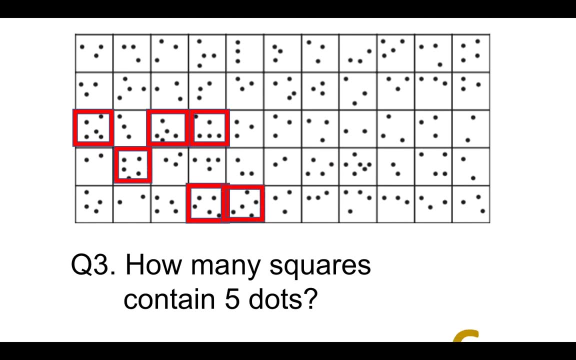 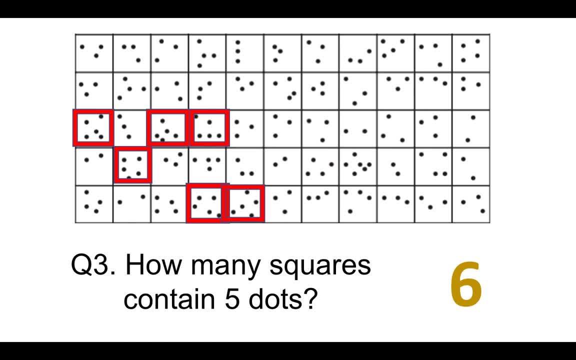 there is six. Did you get it all correct? Please put in the comments section below whether you got that right. Okay, Next one. This is a toughie, so brace yourself. Question Number Four: and again, you've got until the timer runs down to the first three dots. Do you get? 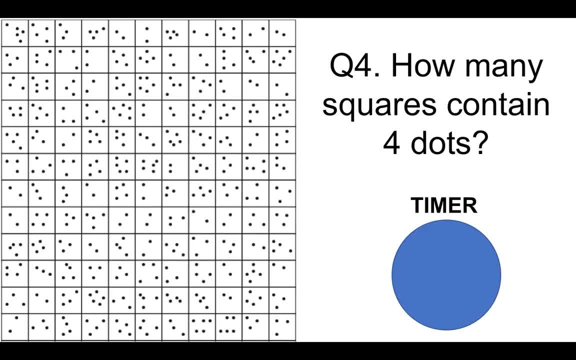 it all right. Please write it in the comments section below. This is a toughie, so brace yourself. Question Number Four: And again, you've got until the timer runs down to answer this correctly. Question number four is: how many squares contain four dots?